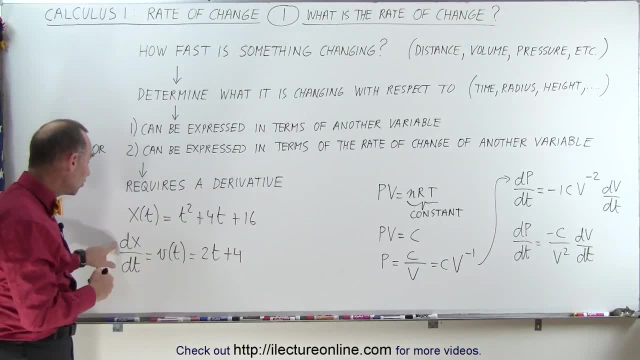 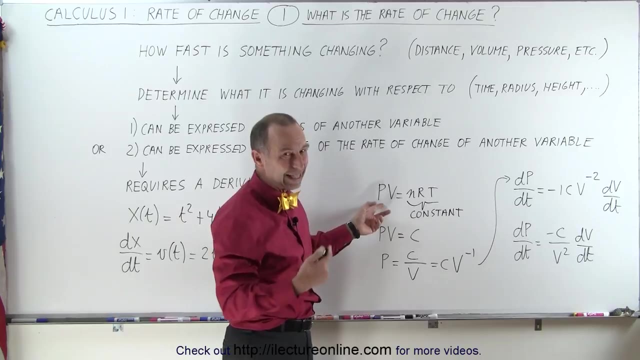 So we can clearly see here that the rate of change of the position with respect to time is a function of time itself. Give me some time and I will tell you how fast the position is changing. Or we can look at an example over here where we have the gas equation, the ideal gas equation. 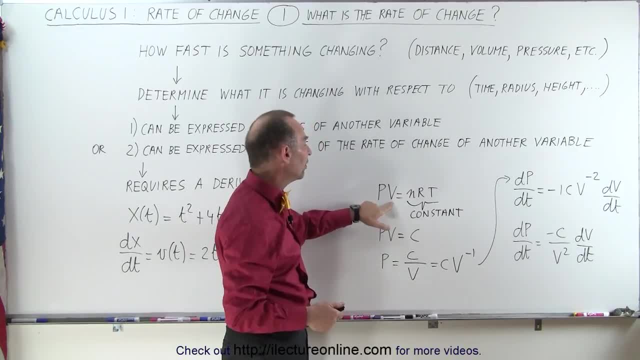 PV equals nRT, where P is the pressure, V is the volume and T is the temperature, N is the number of moles And R is the gas constant. Let's say for a moment that the temperature is constant. We call that Boyle's law. 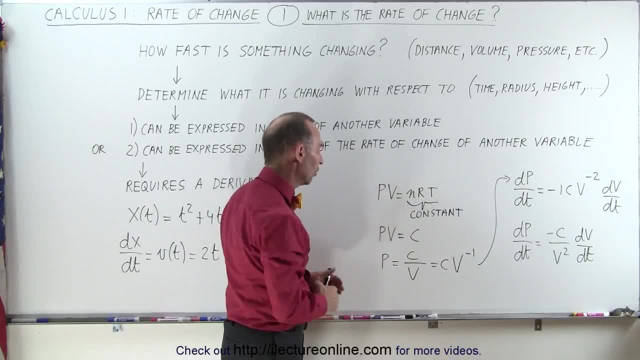 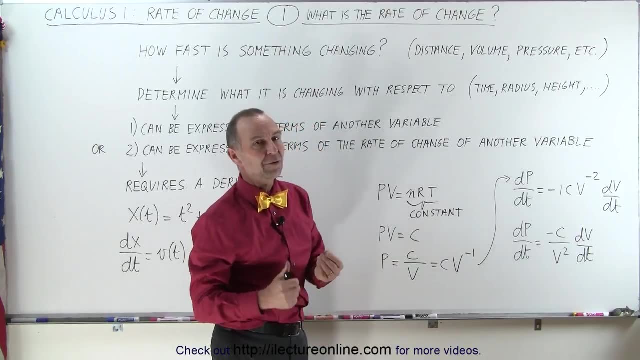 That means that the pressure times the volume is equal to a constant, Or the pressure can be written as the constant divided by the volume, or the constant times V to the minus 1 power. If we now want to see how pressure changes with respect to time, we take the derivative. 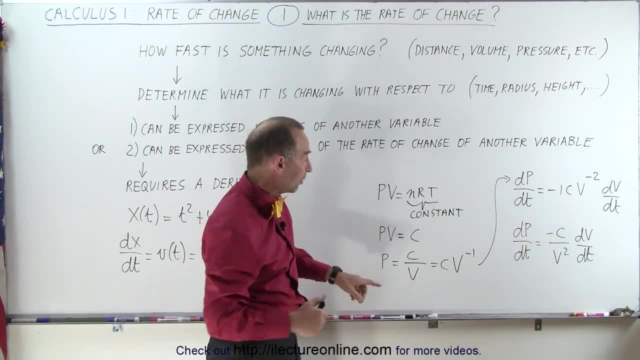 of that equation with respect to time. When we do that, we get the following: When we take the derivative of this with respect to time, we get the following: When we take the derivative of this with respect to time, we get the following: 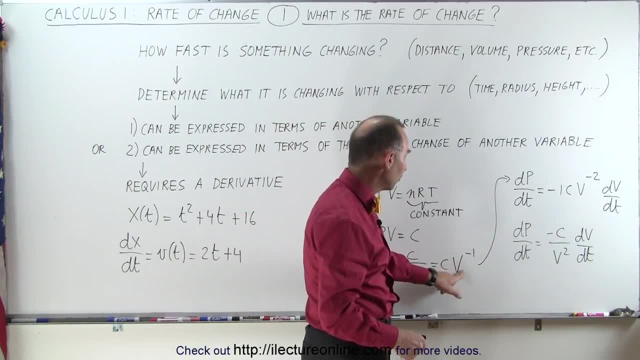 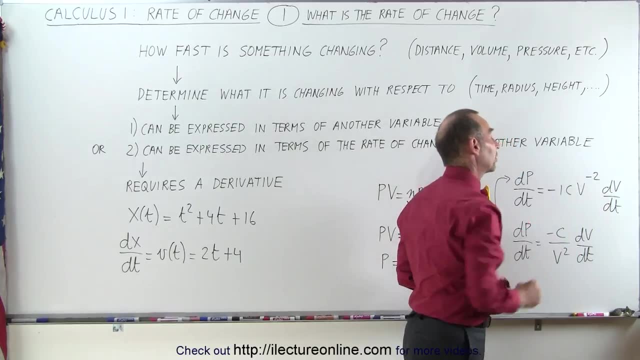 When we take the derivative of this with respect to time, we get minus 1 times V to the minus 2 power, but also times the rate of change of the mass or the volume with respect to time, Because we have also take the derivative of that variable V. 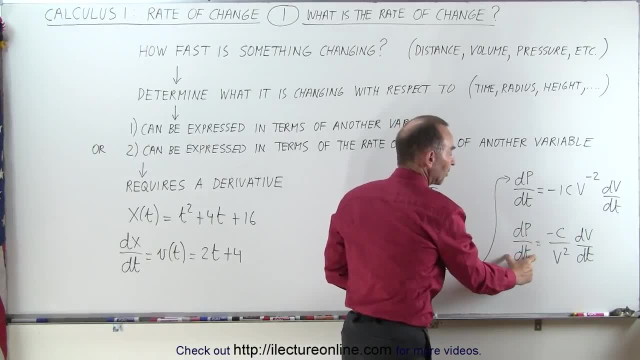 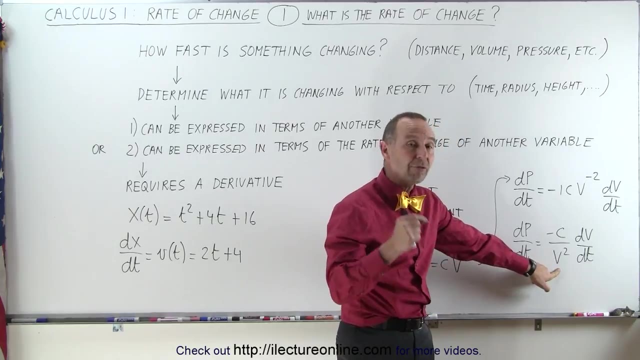 So then we can say that the change of pressure with respect to time is equal to minus constant over V squared times the rate of change of the volume with respect to time, which means that in this case, Right, The pressure depends on both the volume and how fast the volume is changing with respect to time. 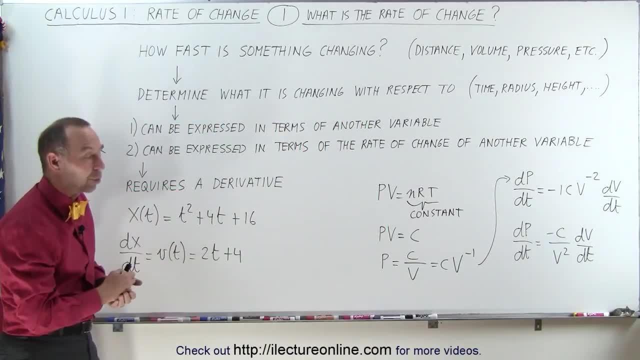 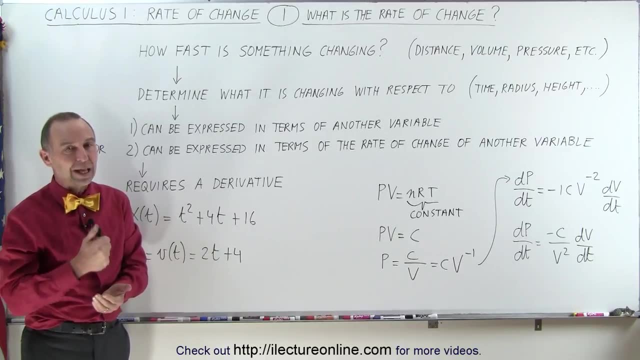 So that's how we can define what we mean by the rate of change, And we're going to look at some examples to help us clarify how exactly we apply that in various situations. And that's how it's done.